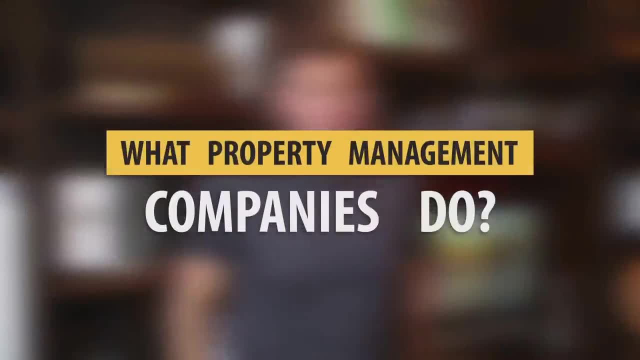 What is a property management company and what is it that they actually do? If you're going to play the game of real estate, you need to really understand this very concretely. So in today's video, I'm going to break it all down for you. 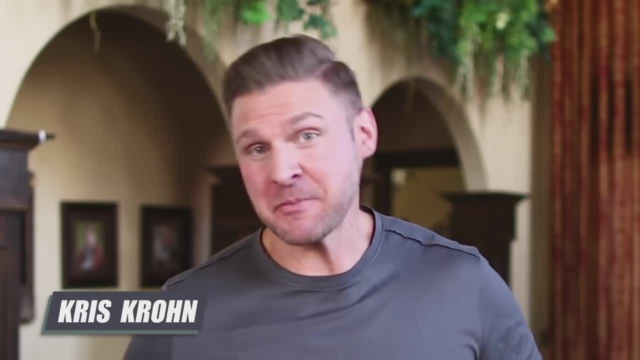 Alright, my friends, Kris Krohn, here and today we're talking about property management. If you're in the game of real estate, you're going to have to decide: are you going to be your own property manager? Do you hire a different third? 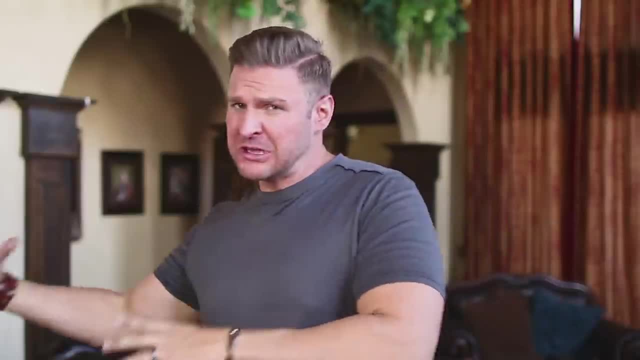 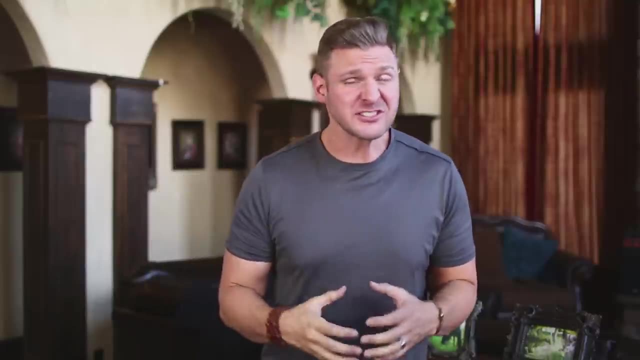 party property manager. Do you skip property management by going lease option? You've got a number of different considerations here and what I want to do is I want to hit the really main big ones for you. that will help you really just understand what property management is. Alright. so the first thing to 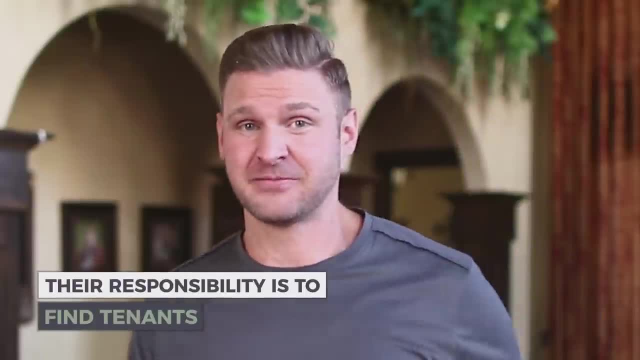 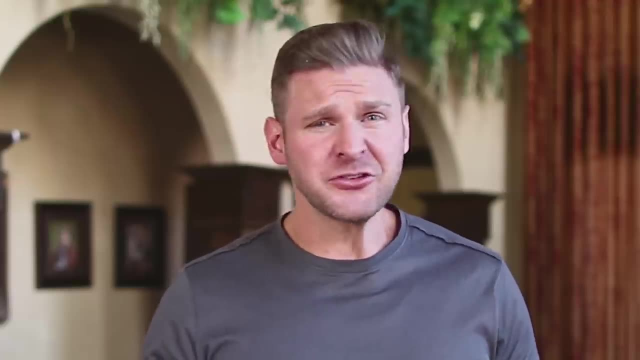 understand is that property management. their responsibility is to find tenants. So if you have a house and it's vacant, you need to get it rented out, then property manager is going to do that. My experience of most property managers is they do not sell lease options. 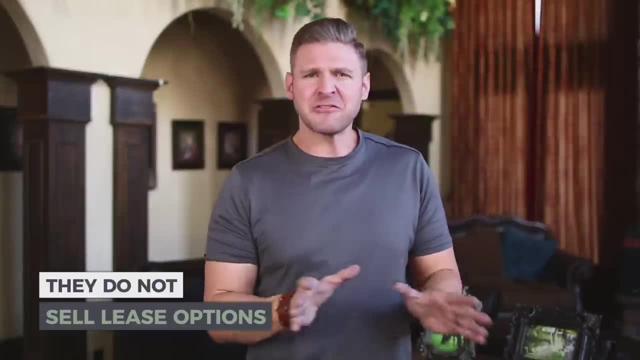 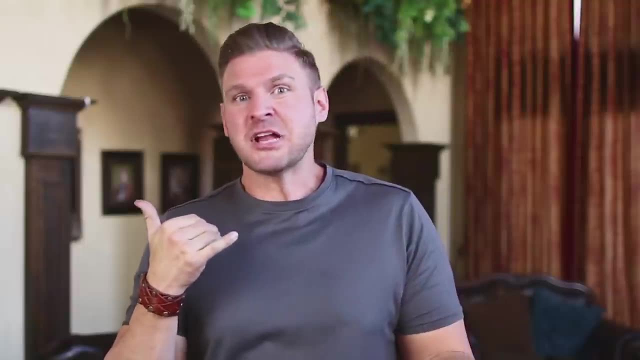 They just do property management. and the reason why that's kind of a big deal is because you might say: Kris, I love your lease option strategy, but if you call up a property management company, 99 out of 100 are going to say: huh, that's not. 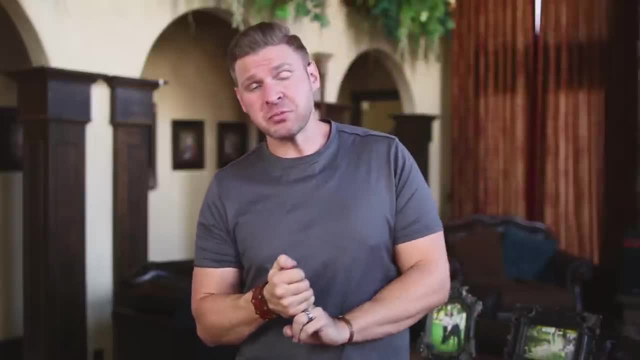 really our bread and butter. it's not really what we do. They will find you tenants. they will also replace tenants, okay. Now the other thing that's really important is they're going to collect the money If you are a big hearted. 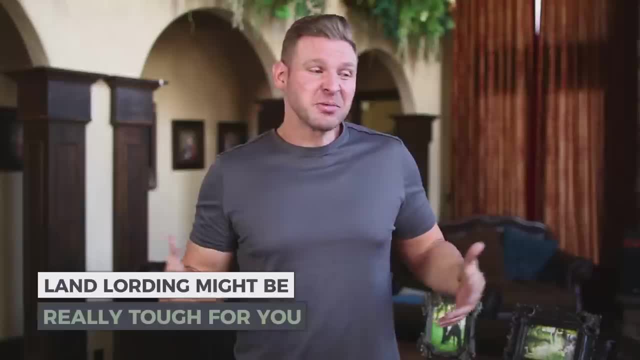 person landlording might be really tough for you because people are always looking for where they got the wiggle room. so a number of people are going to see if they can mooch a little on you, and if they can mooch a little, they're. 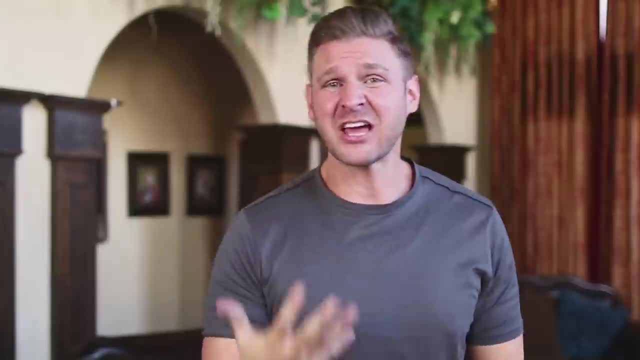 going to take the pinky, they're going to take in the whole body, because that's kind of what goes down. The last thing you want to do is get in a relationship with a tenant where you're in the perpetual habit of being late, so they're. 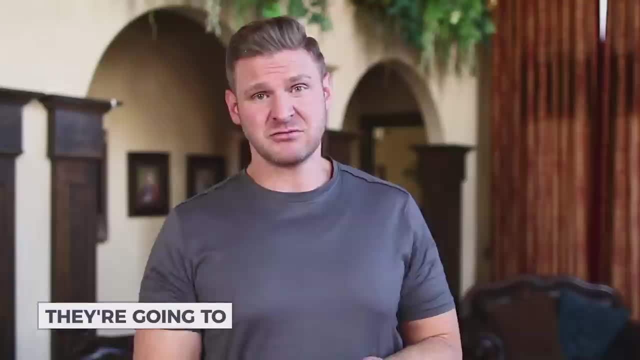 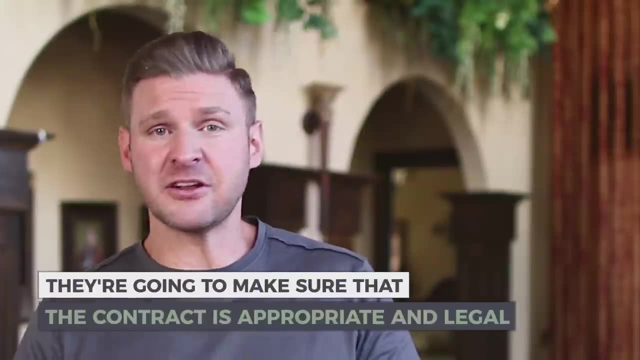 going to go ahead and take care of collections but also take care of fining. They're going to enforce the contract right- If the people are late there could be some late fees- and they're going to enforce and make sure that the contract is appropriate, that it's legal and that the moment anything 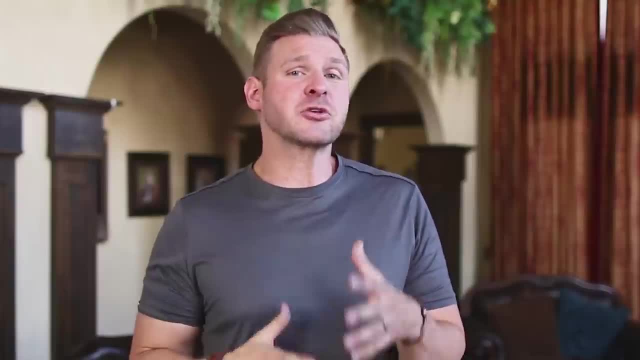 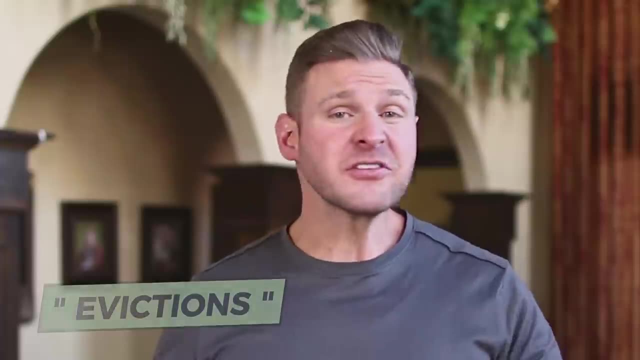 is broken. we're erring on the side of justice instead of mercy, to make sure that the investment goes according to plan. They're also going to take care of evictions. You're going to have some if you buy enough homes you can experience. 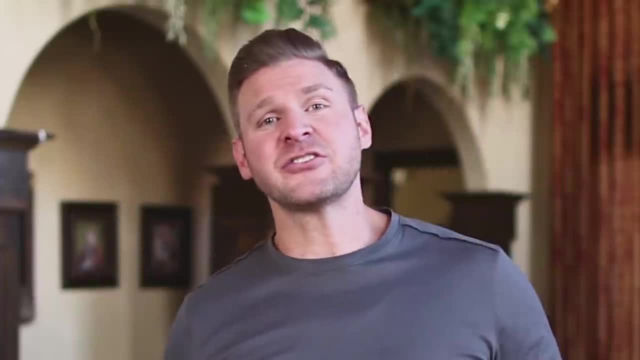 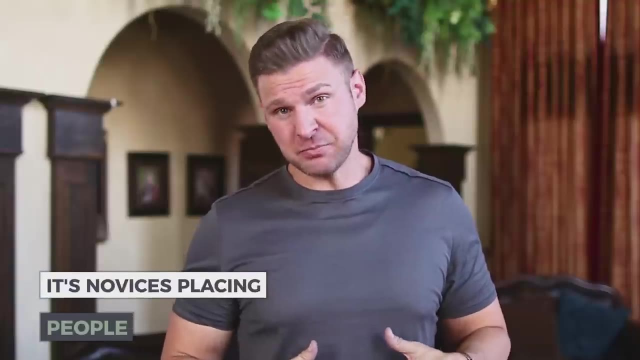 eviction. I know there's a lot of people worried about nightmare tenants. You know where most nightmare tenants come from. It's not property managers placing people, it's novices placing people. so we'll actually put the wrong people in our homes and then when we get what we deserve, We didn't know, but we didn't. 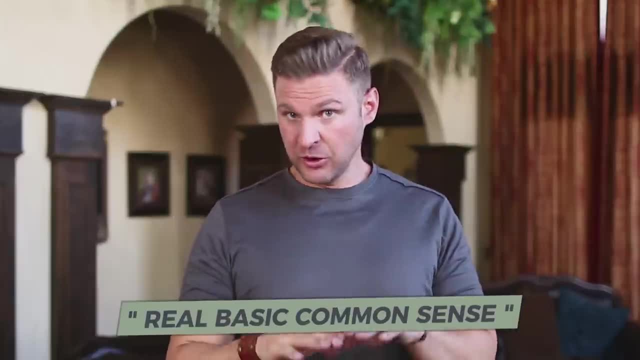 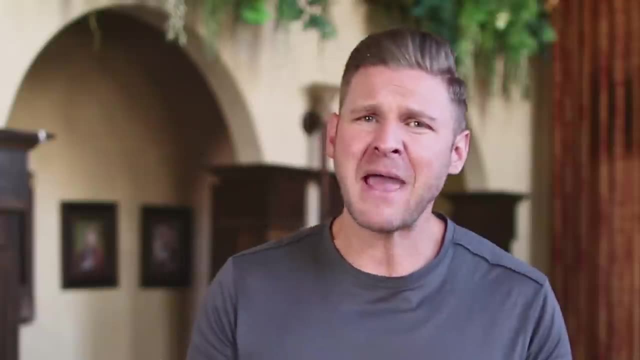 know the standards, we didn't know the mark and the reality is real basic common sense. Hey, this person makes $30,000 a year, but they want to rent this place at $1,500 a month. Well, do some basic math. 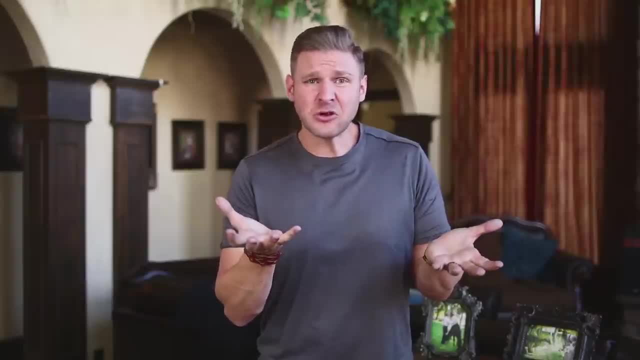 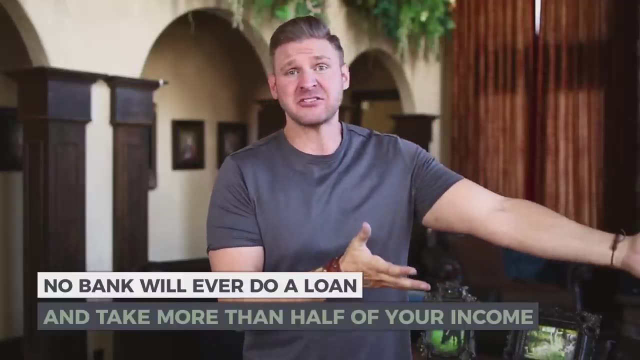 there $1,500 a month. that's what is that $18,000?? That's half, more than half of the money that they make. No bank is ever going to do a loan and take more than half of your income and apply it to your ability to pay a mortgage. So you 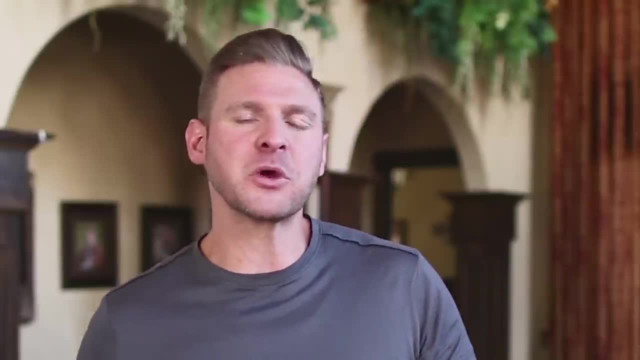 shouldn't either, These property management companies? they have standards for knowing what a good tenant will be, what a bad one will be. They're going to do background checks. they're also going to pick up the phone and they're going to do. 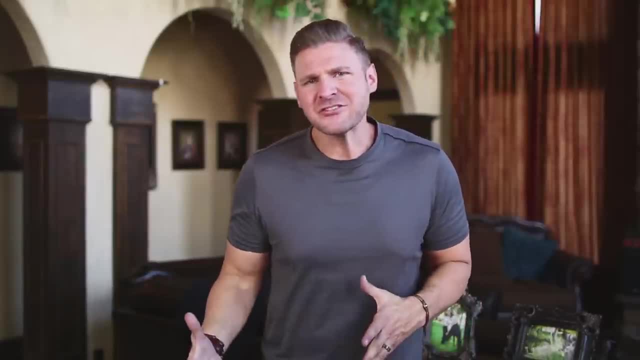 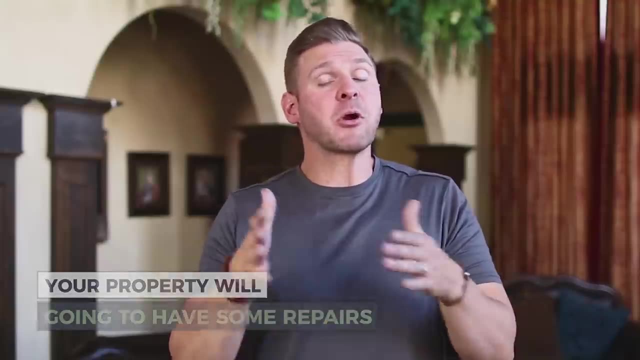 some reference checks if they're a good, thorough property management company. And then the last thing is that your property's going to be a good property. You're going to have some repairs and if you had a property manager involved, they may be the repair company, they may be third party to the repair company and 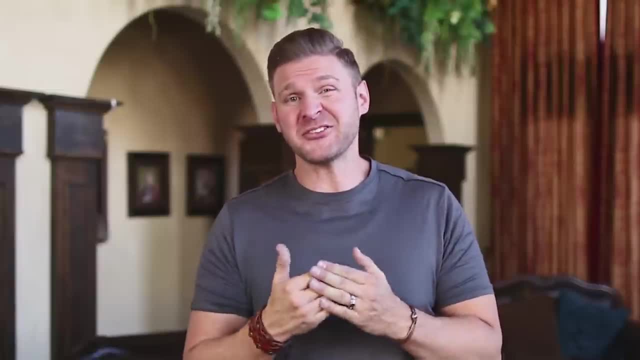 generally, if it's over a certain amount of money, they will send an email, say: hey, this is the bid, this is what's broken, this is what we need you to authorize, and I do get a little skeptical here, just between you and I. 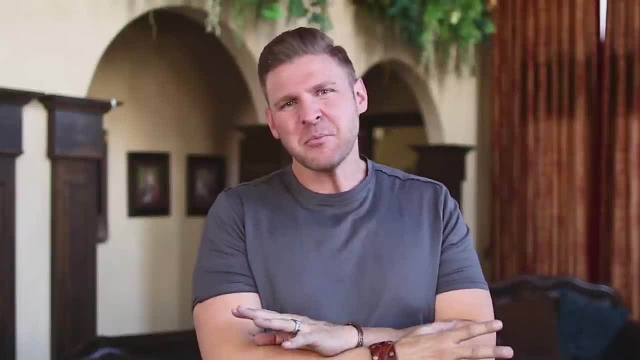 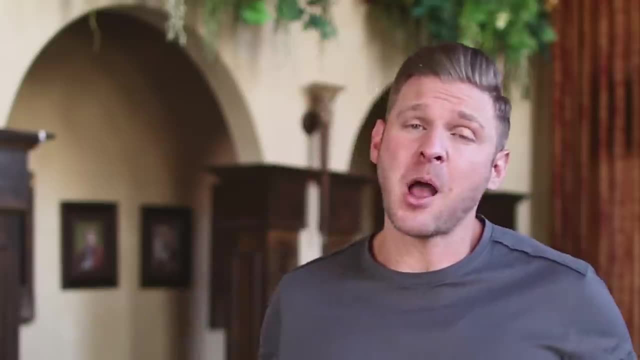 because it's really hard to track a world where there's kickbacks but it's not like the property manager is trying to save you money. So often they'll go to super competent repair people, but the super competent might charge you double or triple. so that's where you might want to get a little bit involved when it 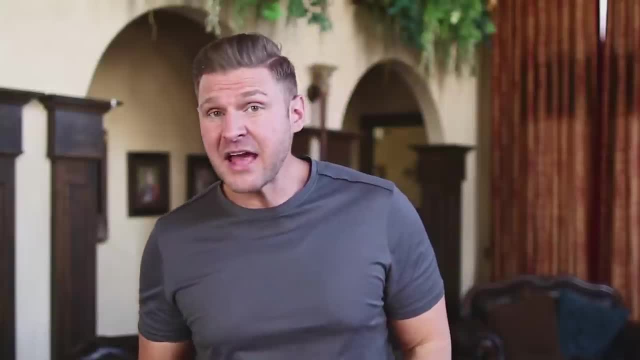 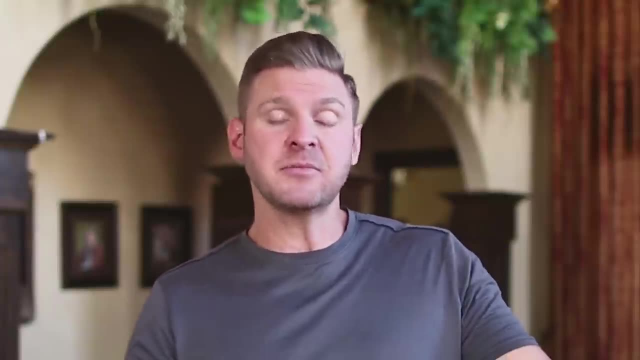 comes to approving the repairs of the property. but outside of that it is nice. it can be totally headache-free. something breaks and they're going to take care of it. If it's over a certain amount of money that you set up with them, they're going to make sure that they get your buy-in and approval. so 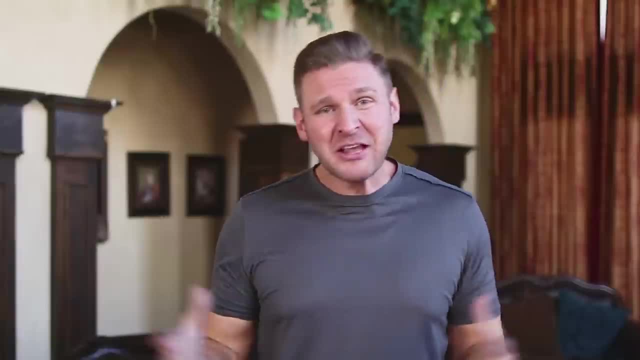 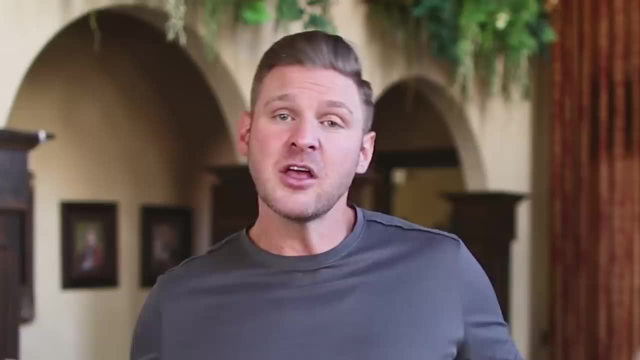 there you have it. Property management, in a nutshell, A to Z, soup to nuts- is basically: they're there to find people for your house, enforce the contract and get people out if they're the wrong people and otherwise they're going to do. all of that and charge you roughly 10%. Some might charge 9,, some might 8,, some might charge 12, it depends, but 10% is really an average amount that they're going to charge of your gross rent. So if you're renting a house for 1200 a month. 10% is going to be $120 a month. That's what it's going to cost to have them. and I'm going to tell you right now. if you've got an awesome tenant in the house, then you'll be like: why am I paying this?